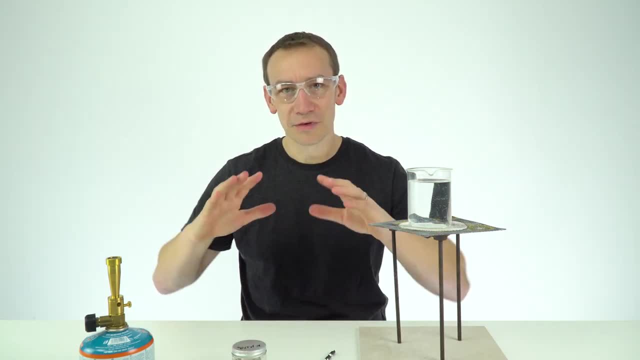 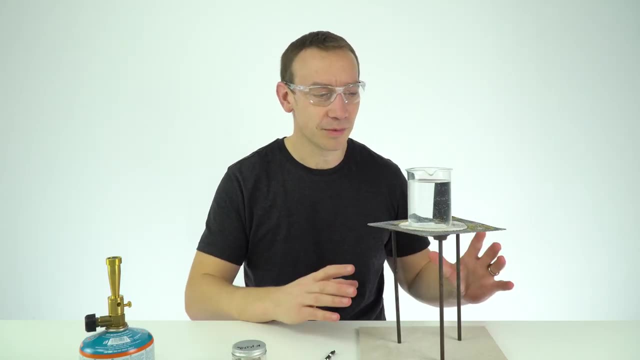 throughout. The other thing I'm going to make sure is I'm not sat down at the desk, because if we were to have some hot water in this beaker and it fell over, if I was sat down I couldn't necessarily move out of the way. so I'm going to be stood to one side of the beaker and I'm going to 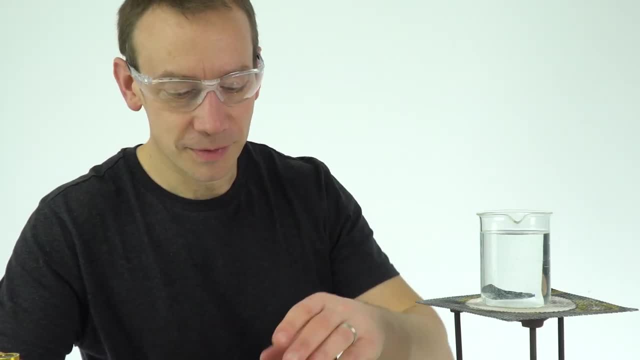 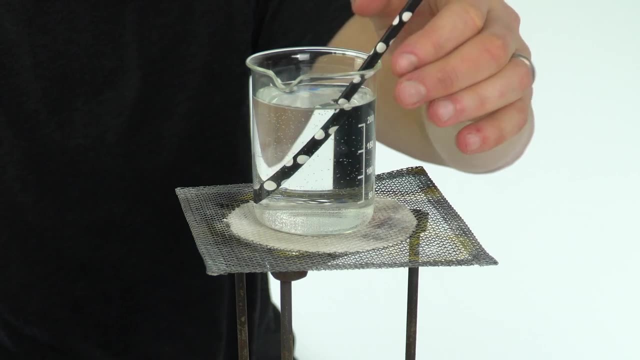 be on one side as we're heating this up. Now, in order to get this potassium manganate to the bottom of that container, I'm just going to use a straw. so if I just put that in there very carefully, I'm just going to get a couple of crystals of this and put it down to the bottom. You don't want to. 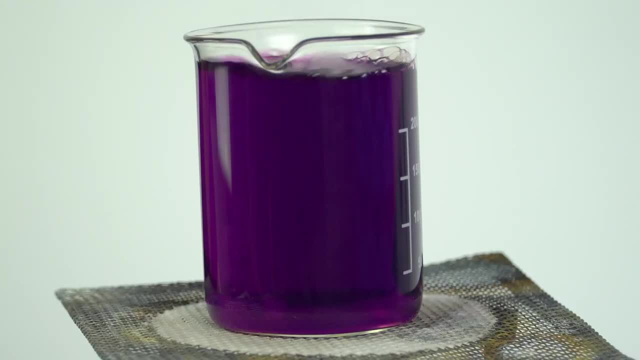 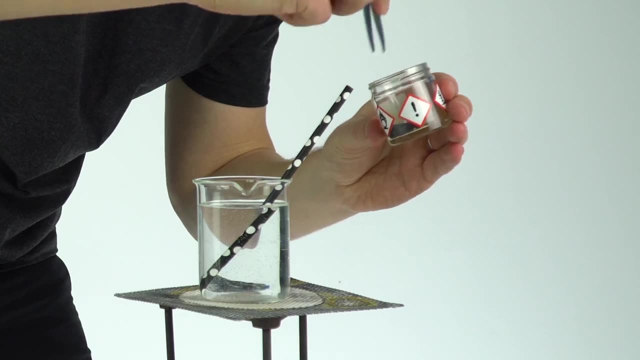 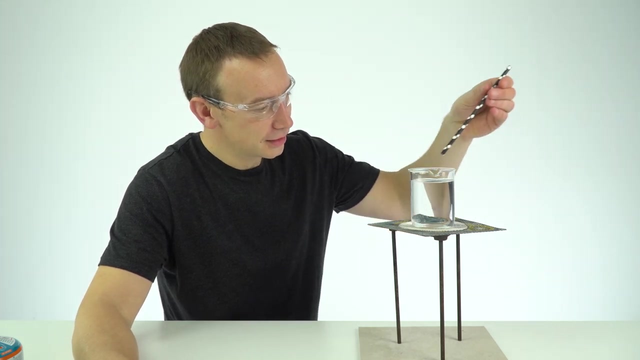 be putting loads in. otherwise, all you do then is you end up boiling purple water, and that doesn't really show anything. so, in a way, less is more. So I'm just going to add a few crystals. Now, I've just put literally one small crystal at the bottom, hardly anything at all. What I'm now going to do is I'm going to 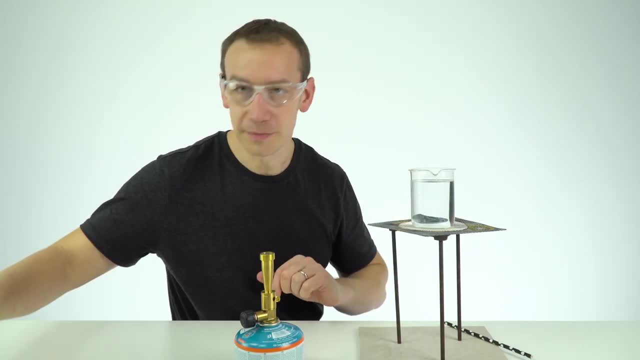 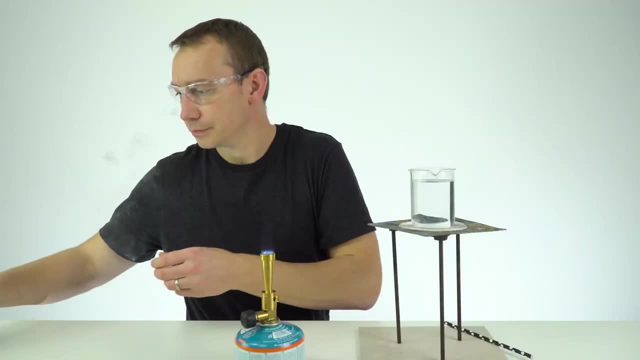 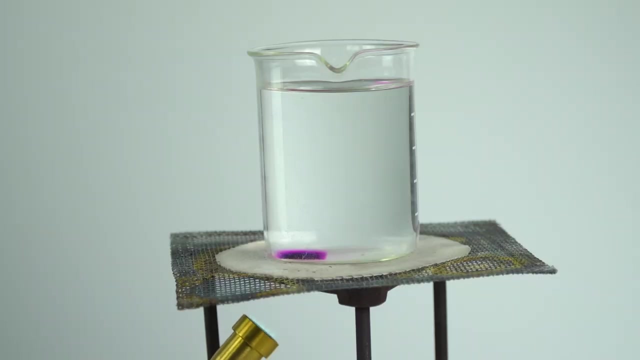 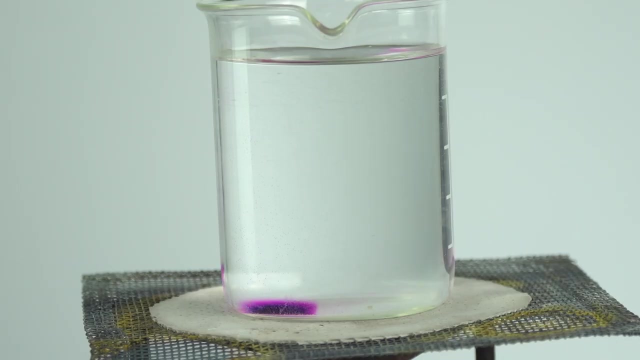 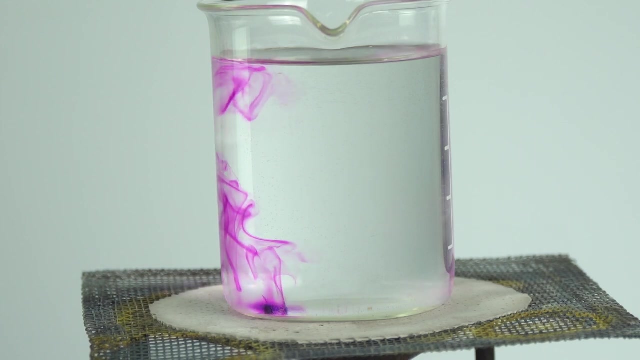 light the Bunsen burner and just very gently heat on this side of the beaker. We can now see how the water is rising up above that crystal and then, when it gets to the top, we get this current where it maybe starts to move down the other side as well. What we now have 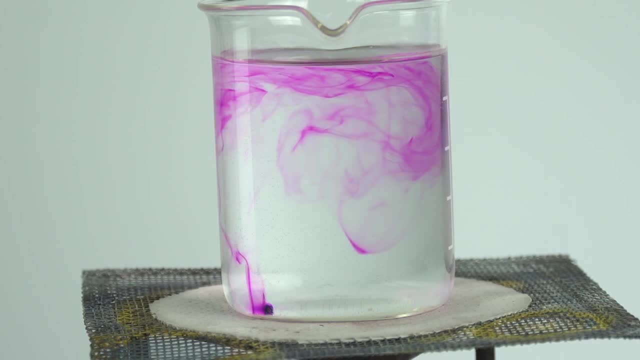 inside the beaker is a convection current. We're going to just heat that for a few seconds and then the water will keep moving all the way up to the top of the beaker. What you're going to do is you're going to heat this with a steamer so that you can fully heat this beaker up. 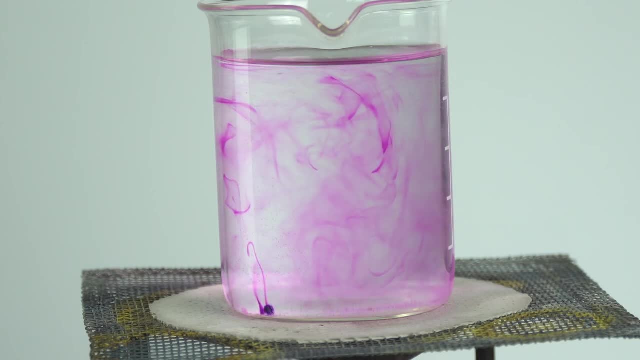 Now we're going to heat up the beaker a little bit and then we're going to just heat it up. So if you look at the beaker in the middle, you can see the water's already started to boil, and then one of the crystals is going to start to boil down just a little bit more so that the water gets to it. 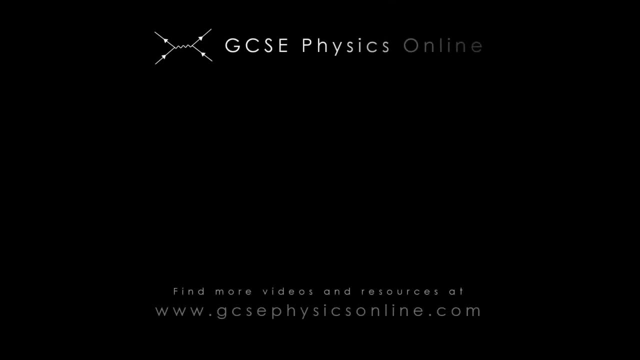 You just keep heating it up. Thanks for watching.